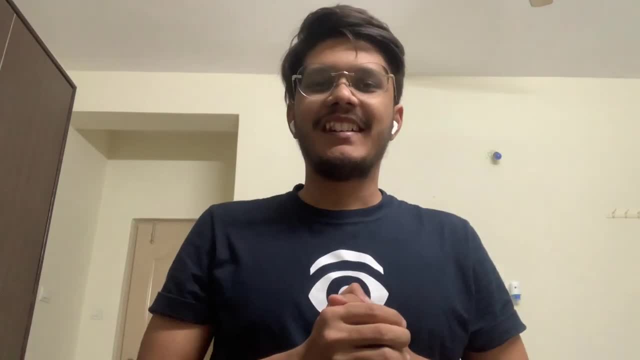 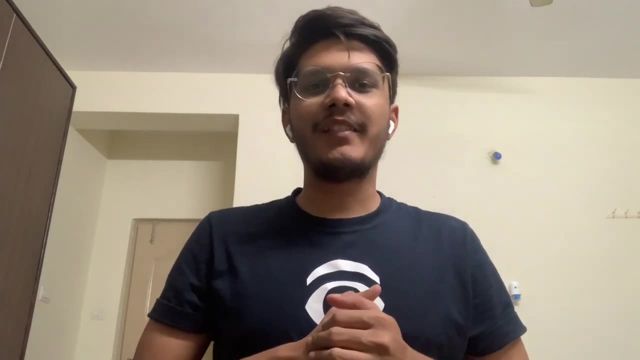 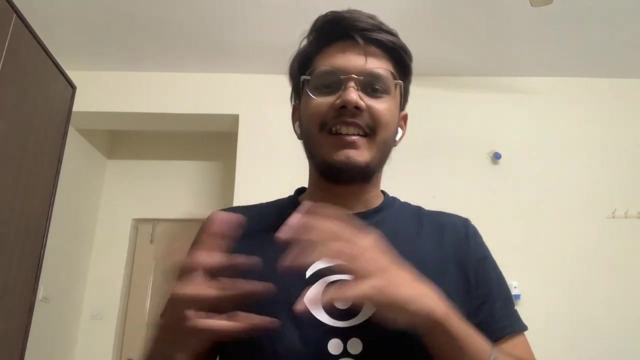 Hello everyone, I am Ashwin Kulkarni, welcoming you all in this Quantum Computing Learning Gen. I hope you all are doing well and learning something new everyday. I apologize for the delay, that this video is coming out very lately compared to the last ones, because it was my 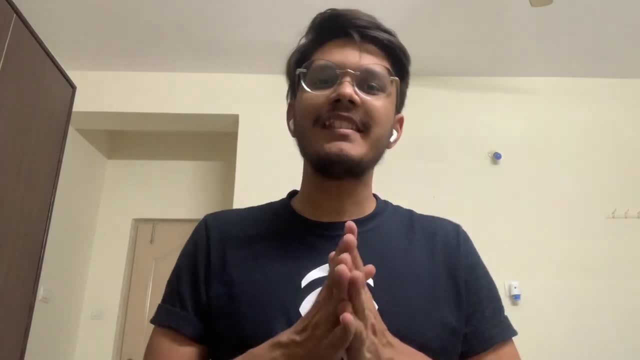 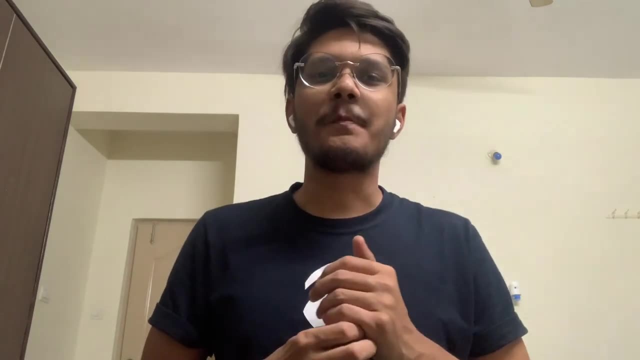 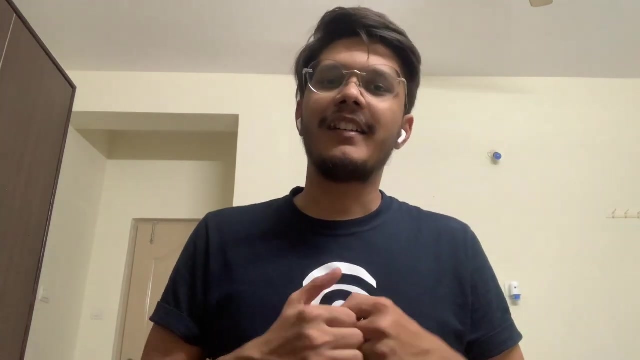 some personal stuff is going in the back behind the scenes, But yeah, I'm back with the another video. So in the last video we have seen the single qubit gates of X, Y, Z, Pauli gates. Now in this video we are again continuing with the single qubit gate, but a special one. 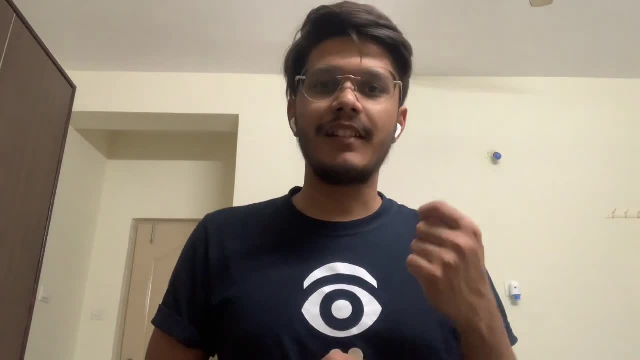 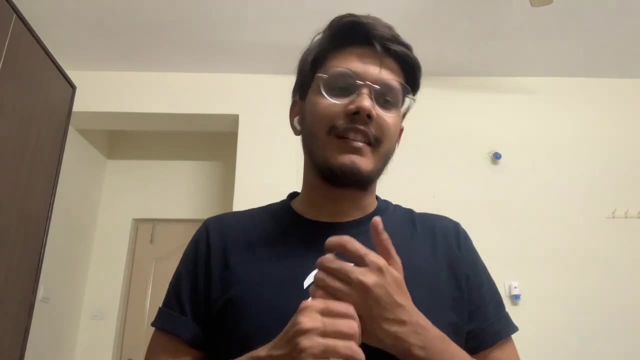 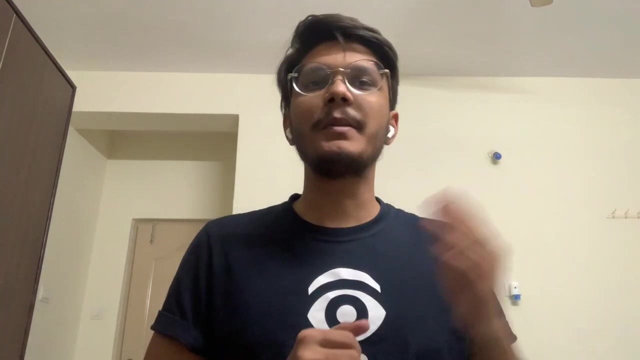 where, with the help of that, the superposition happens, and all that buzz around the quantum computers, which is the superposition, This, this particular gate, is the basis of that which is head, market or educate. So in this video we are going to talk about that and we are going to learn. 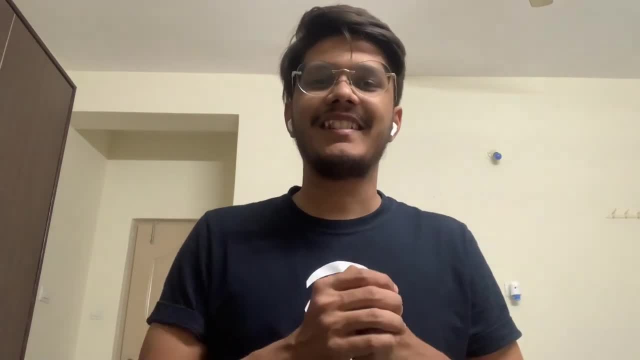 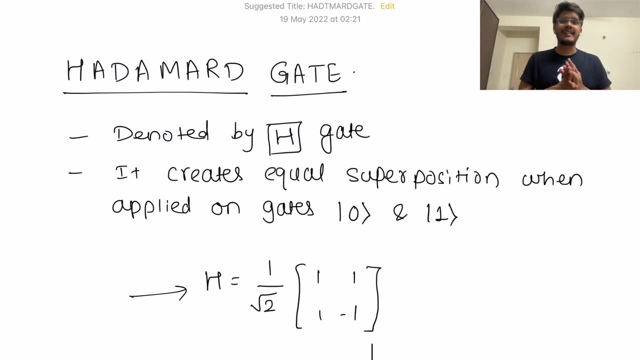 about more about it. So let's get started. So since the beginning, we have been talking about the superposition state in the quantum computing. Now, what is very special about it and how to make your normal state to a superposition state? That's what we are going to see in this, in this part. So a superposition. 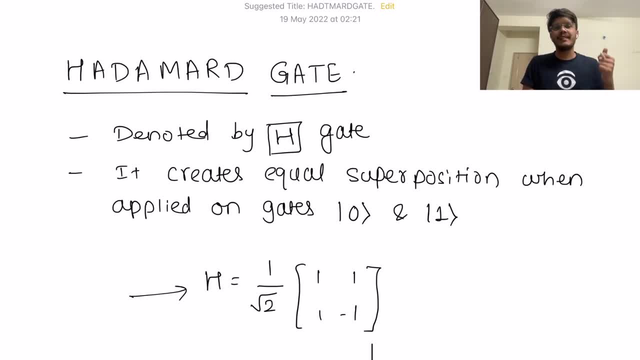 state where your quantum, your very qubit, can be into a multiple state by having a different probabilities of being into different states. So the head market is the basic gate useful for the superposition operation. Now how head market is important? Because your basic State 0 or basic state 1 will get transformed to a superposition state. 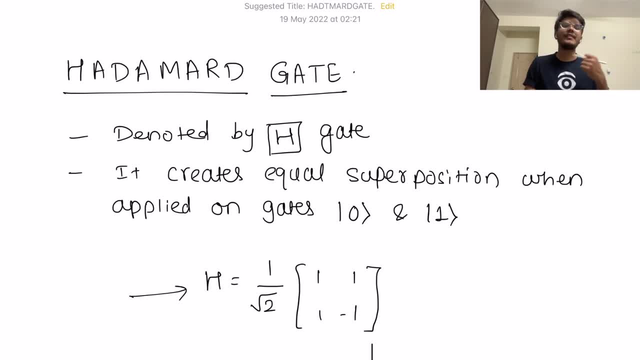 by applying head market to it, And that's why it is getting used widely into quantum systems where the superposition is the crux of it, And that's why head market is very, very important in this whole journey. Now the head market is denoted by H, So various 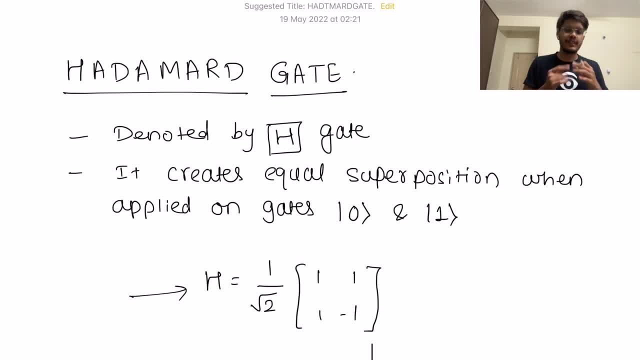 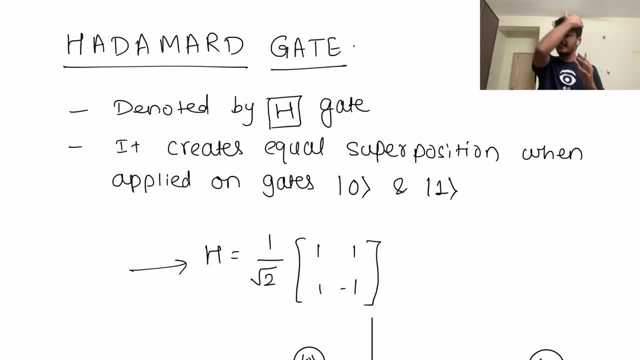 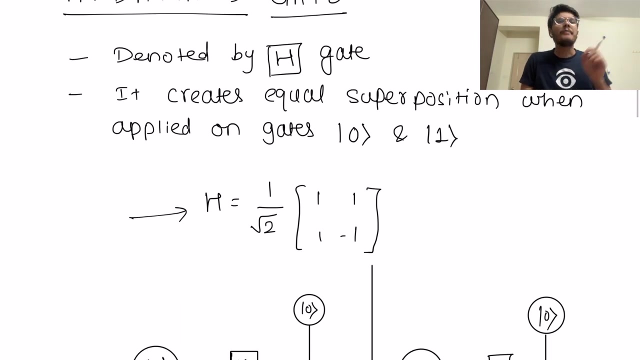 in the in IBM quantum lab or wherever you see the H symbol in the quantum circuit. that represents the head market and, as I already explained that, it creates the equal superposition when applied on the gate 0 and gate 1. so equal superposition, as in it, will be in the state 0 and 1, here with the equal probability. now the 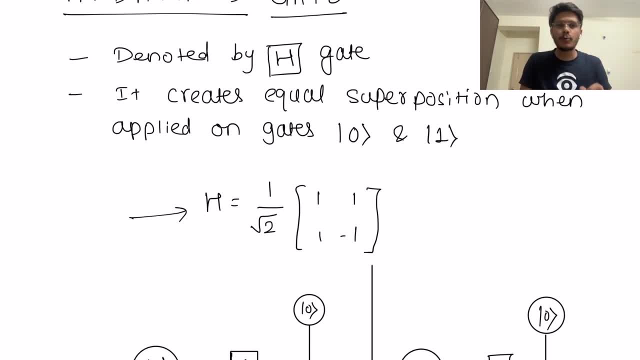 head market is defined by 1, by root 2 of 1, 1, 1 and minus 1, so this will be a 2 cross 2 matrix, same as XYZ Pauli gate, how we have defined. similarly, the head market will get defined now, as I already explained, your zero gate will get. 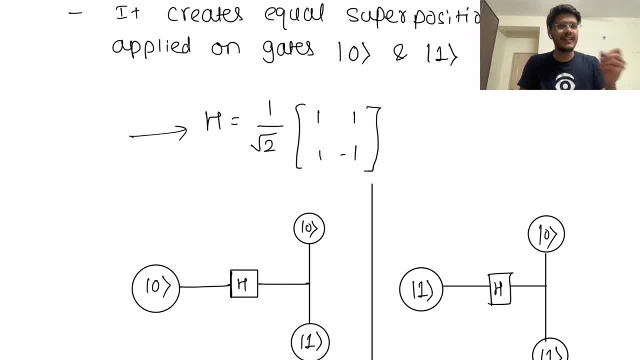 transitioned into the state 1 and state 0 similarly by a, by applying the head market and, similarly, or state 1 will get transitioned to state 0 and when? so what that means? then, by applying head market to your state 0, it will get superposition to some other state where it will be in the state 0 as 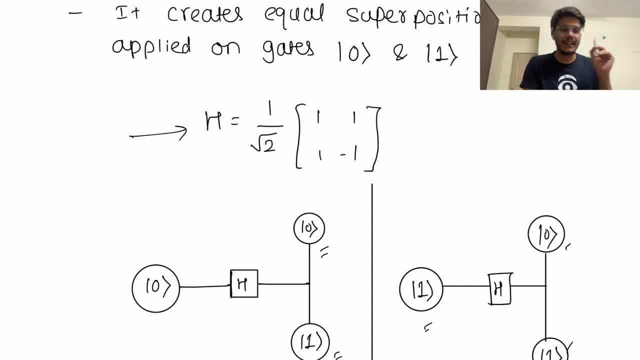 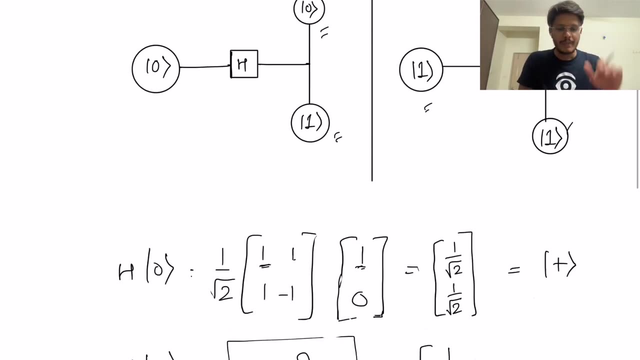 well as in the state 1, and similarly, by applying head market on the state 1, qubit having state 1, then it will get escape phase, will get again transition to state 0 and state 1 at the same time. now how, how this happens is, you know, when you apply head market on the zero state. so 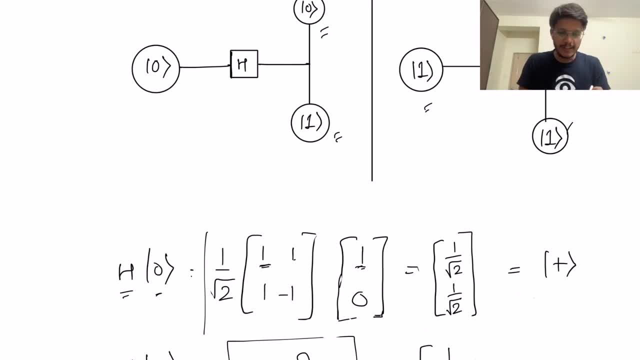 mathematically, we are going to see this scenario. so this is the head market equation, right, as you already seen? now, this is the zero gate, zero gate matrix. so when, when? so this is the gate matrix. when this gets applied, so this one will get multiplied with this one and this one will get 0. so that's why you see the 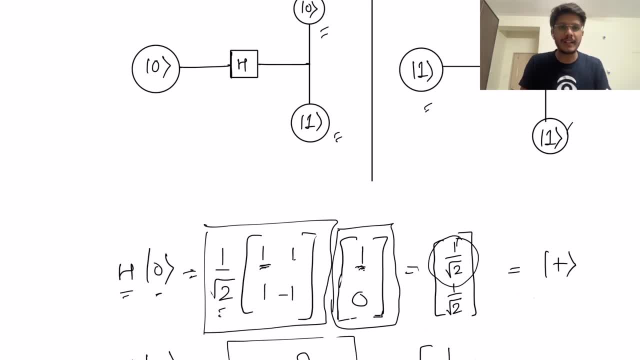 1 by root 2 here and similarly, this one will get multiplied with the first one and minus 1 will get multiplied with 0 will get cancelled out. so you can again see the 1 by root 2 now. the first one by root 2 represents the state 0 and the 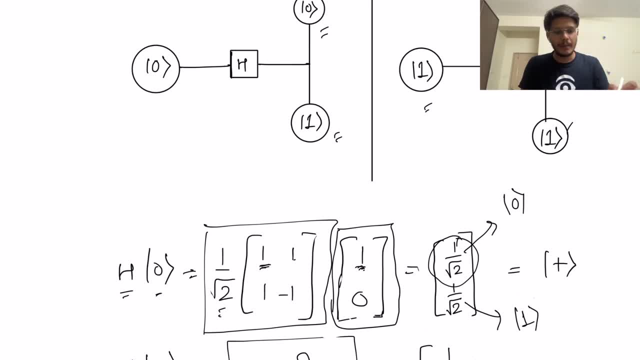 second one represents the state 2: 1, having the amplitudes as 1 by root 2, 1 by root 2. hence the probabilities will be square of these amplitude, hence the probabilities of r 1 by 2. so that means this particular superposition state is 50% in the qubit state 0 and 50% in the 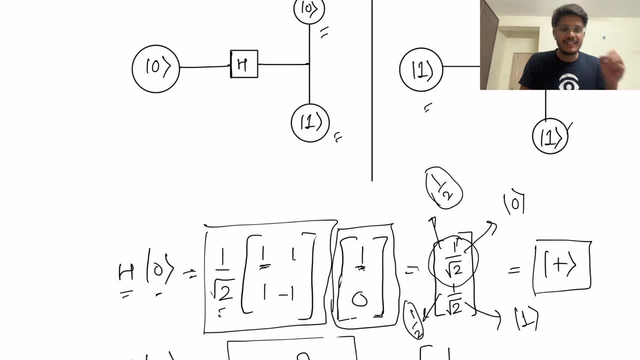 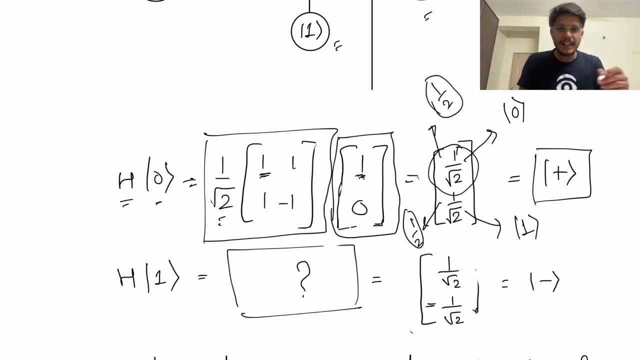 state 1 and that's why this plus state is the special superposition state, having the equal superpositions of 0, equals plus superpositions, having into 0 and 1 state. similarly you can try it out: the mathematical multiplication when H gate gets applied on the quantum state 1 and. 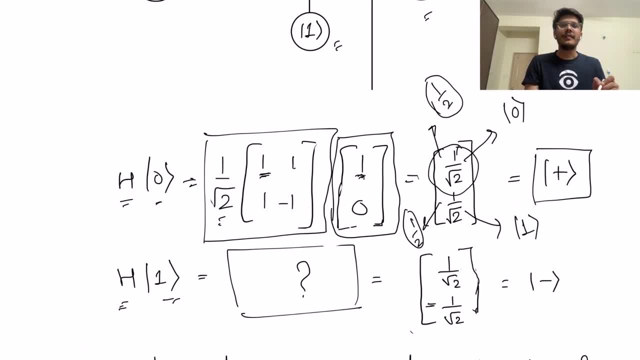 the output will be 1 by root 2, 1 by root 2 of state 0 and 1 by root 2 of state 1 with the with the reverse phase angle. so that's why this is another special superposition state. so these two are superposition states when we apply head. 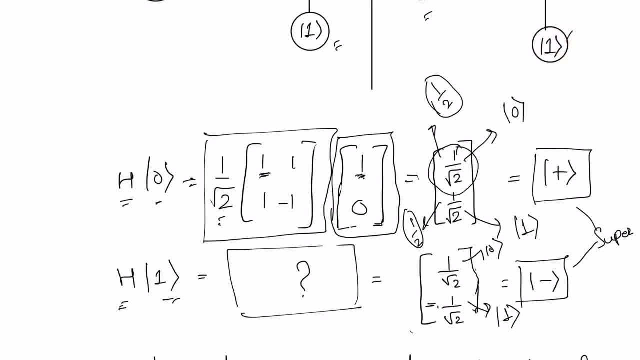 market on 0 and 1 respectively. now the special property of head market is it shows the destructive interference. so what is interferences? basically, it can amplify the different state to make some neurons state. so it can amplify, amplify the input state to uh, to make the some other new state. or it can disamplify the states by 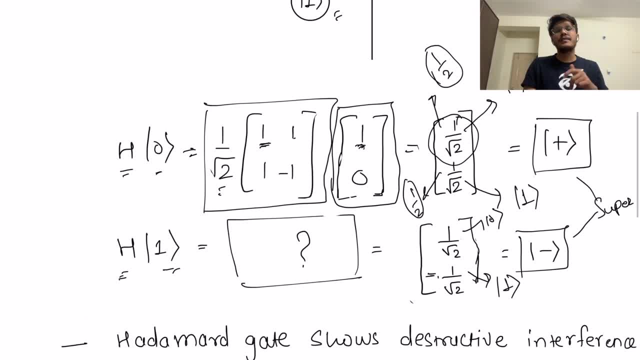 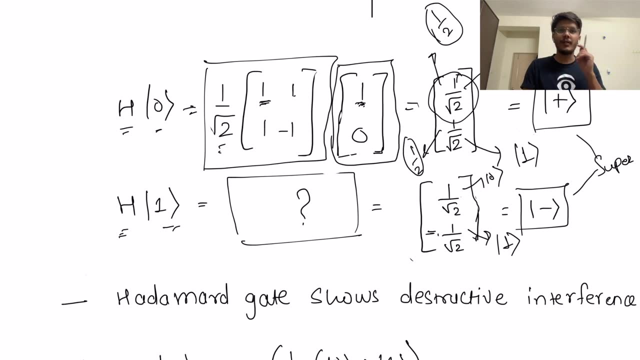 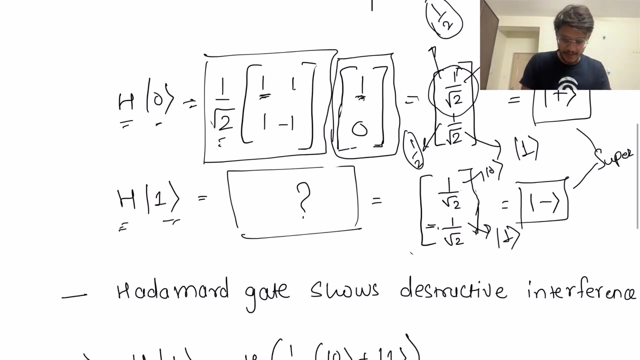 subtracting each other. so the destructive interface means it will get. so different states will get cancelled out, different similar states with um with some opposite properties will get cancelled out. so head mart gate shows the destructive interference on uh on phase, uh on on qubit, state 0 and 1 in different scenarios. so now uh from the first video or 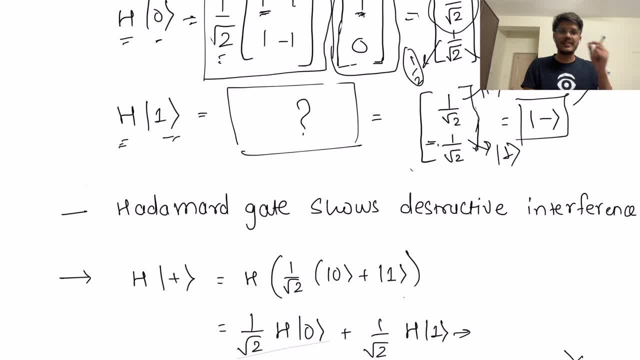 second video i. i already explained that this special property of quantum gates are it is reversible. so that means from the output state you can still get back the input state, unlike the classical states, classical gates- where you cannot get the input states from the output states. but in the quantum states you can get back, and by playing different, of course, different. 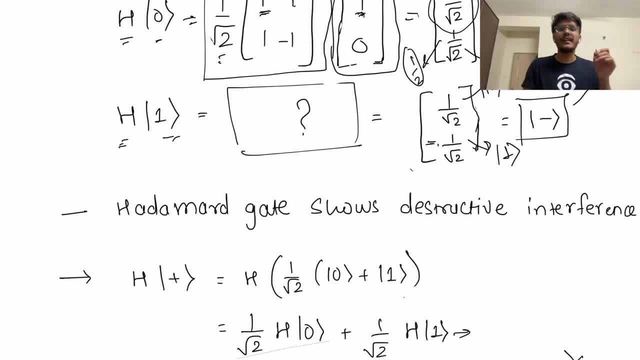 gates and different operations to it. but in case of head market it is so special because if you apply the head market on a particular state you will get some output state and if apply head market again onto that you will get input state. that's it, the two step operation to get. 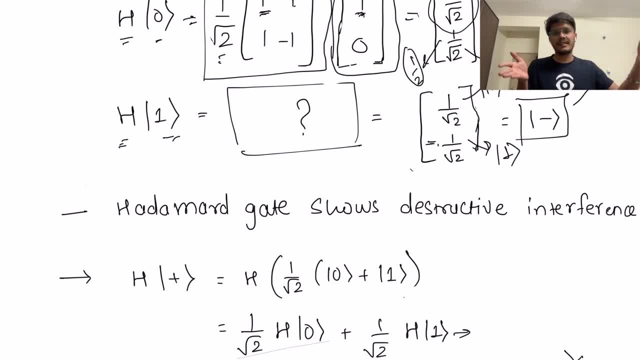 from state input state a to again input state a. so, for example, you you are in the current state a, you apply head market to it, so it will be in the state b, and you again apply head market to it, so again it will be into state a. so these two states are same this way, if you apply so 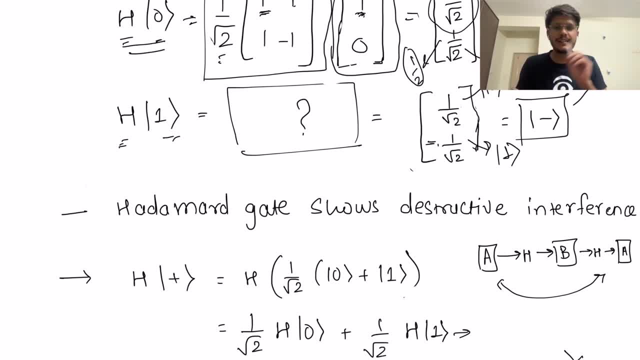 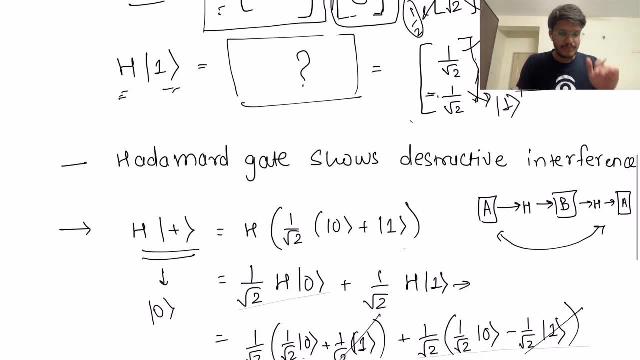 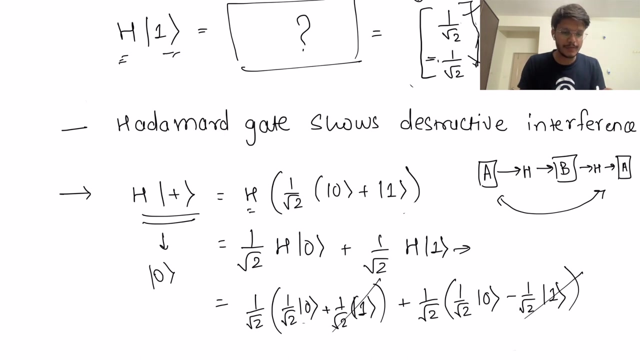 think on it. when you apply head market on the state 0, you have got output as plus superposition state. now when you apply head market on the plus, you should get your zero state back right. so mathematically we are going to prove this. so you are applying head market onto state plus super. 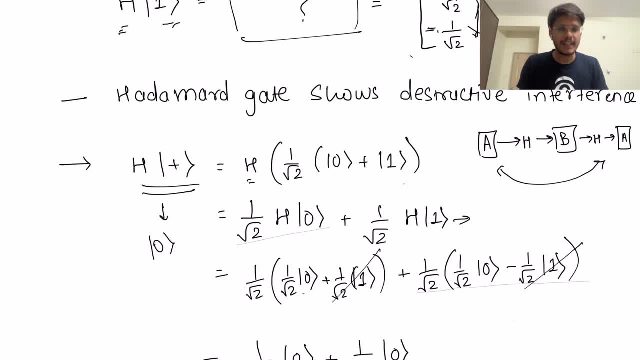 plus, which is superposition state. so, similarly, this head market 2 will get applied to 0 and 1. now again, head mod on 0 will be: this is the plus state and again, this is the minus state. now, in this case, what you do is you are applying the zero state as minus 1, 0, 3, and then you apply: 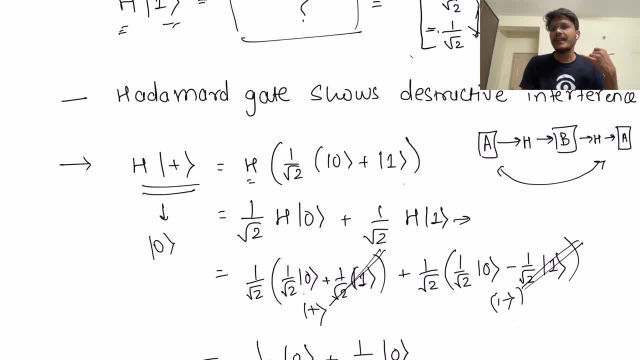 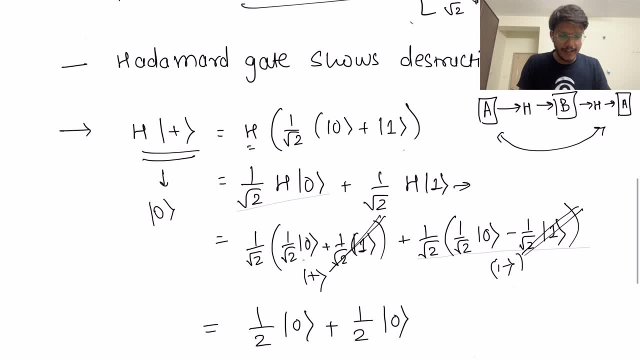 the zero state on the 0 and 1 and plus 1 0, 3, but you will be doing the same thing, so you should apply the zero state on the other side of the base and vice versa. so this is the first step and then you apply the zero state on the other side of the base. so from here you can see that. 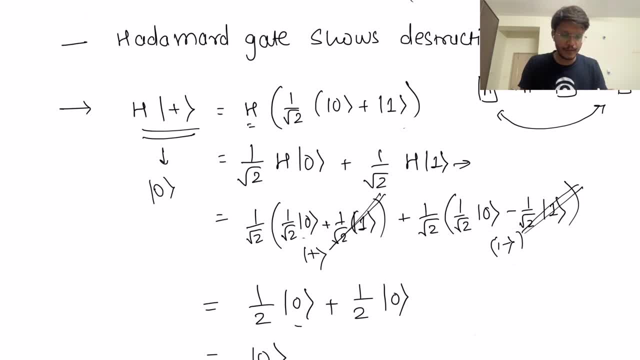 we have already taken that influence of the Jacob's curve, which gives us a few examples so you can understand how this works by looking at this and applying the zero state on this step. now let me just explain on this stage. I'll try to show you how to do this, so I'm going to do this now. 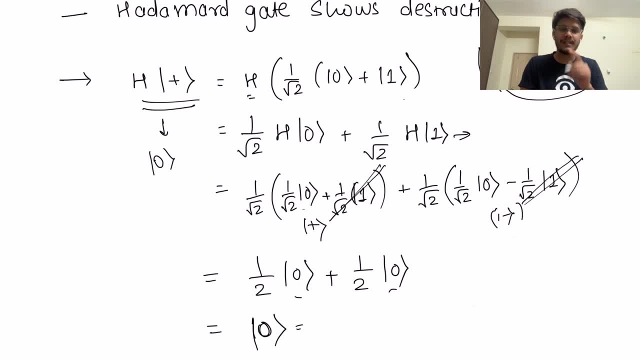 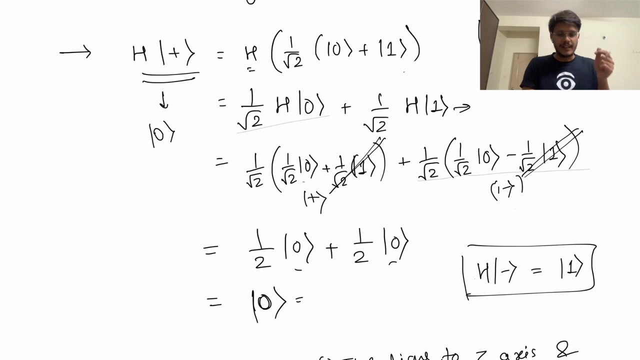 state, which is the original state and that is the special property of head market as well. now the exercise for you guys is to try it out: head marked: applying head market on minus, you should get back state 1. so this is exercise. please go ahead and try this out now. on the blocks pair: how? 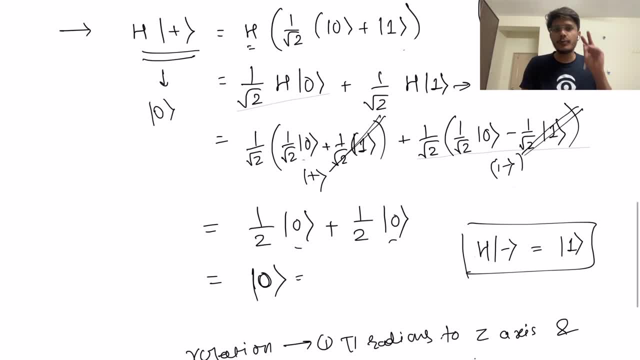 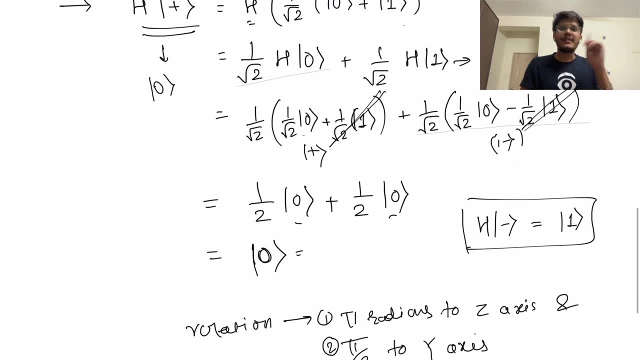 head market works is there are two steps to get the output of any particular state to head match state on the blocks, where first what it will do? it will basically, along this head axis it will rotate the state to pi, pi radians and then along the y axis it will rotate it to pi by 2 radians and that is how on. 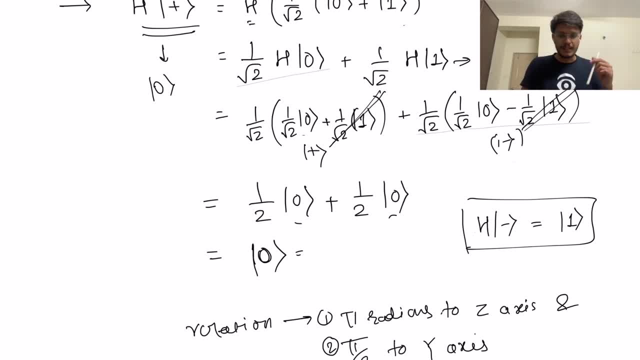 the blocks, where also you can see the output of output of the head market applying on a initial, any initial state. so this is it about the head market and I hope you have got a clear picture about the superposition from this video. we are going to discuss more on more on it, on. 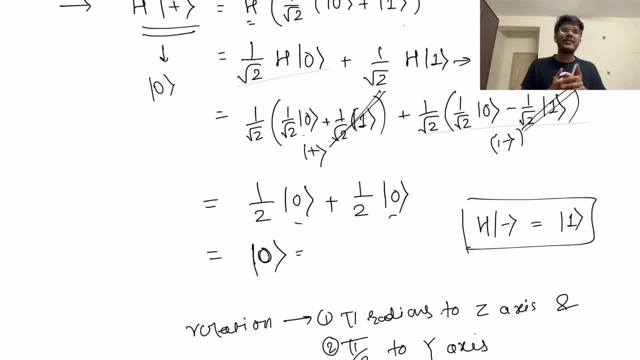 the upcoming videos. so I hope you like this video. if yes, then please give it a thumbs up and share it with your friends and whoever is entering into the quantum computers or whoever wants to learn about it. so please like, share and subscribe to my channel. I hope to see you in the next one. 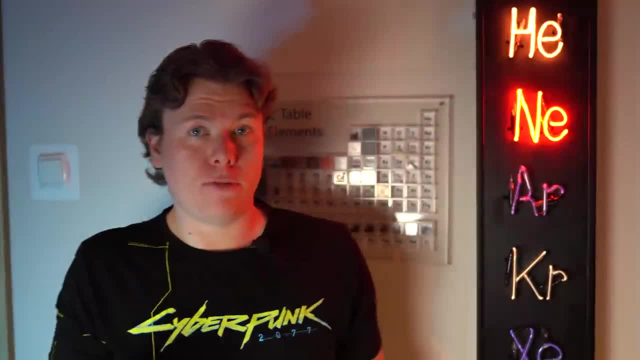 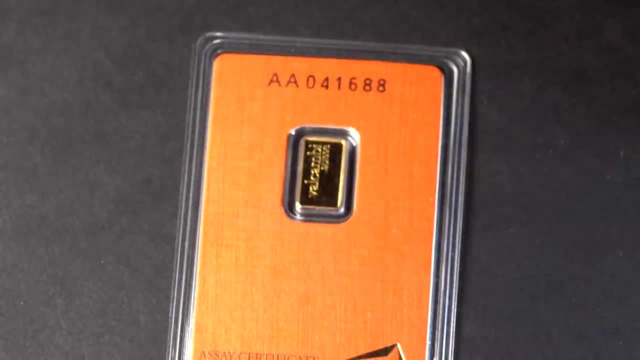 It's true that today, prices of some items, including different metals, are going up quicker than before. of course, to protect your savings, You can invest your money, for instance, into gold, But it would necessary be increasing it worse as rapidly as before, or else it cost may even decrease. 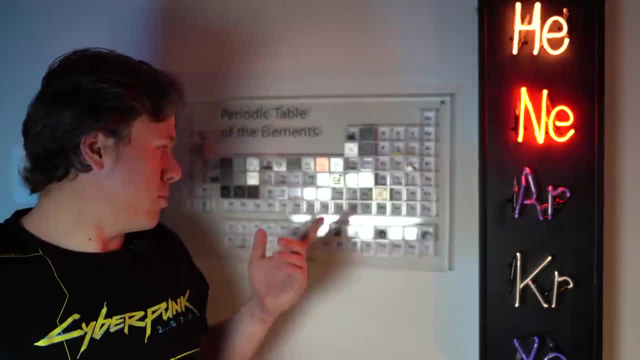 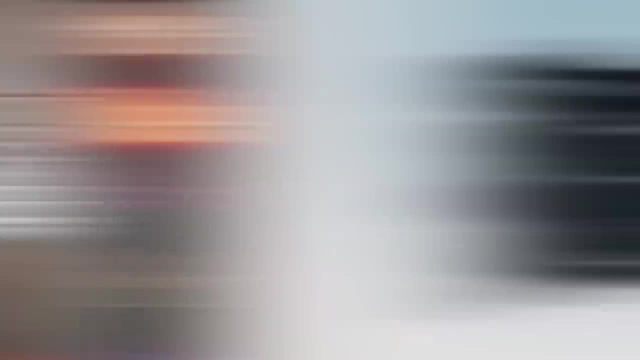 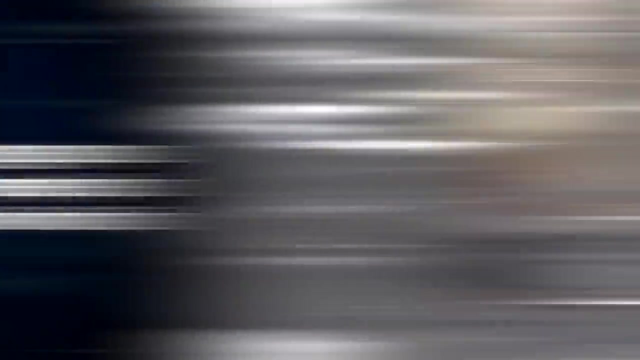 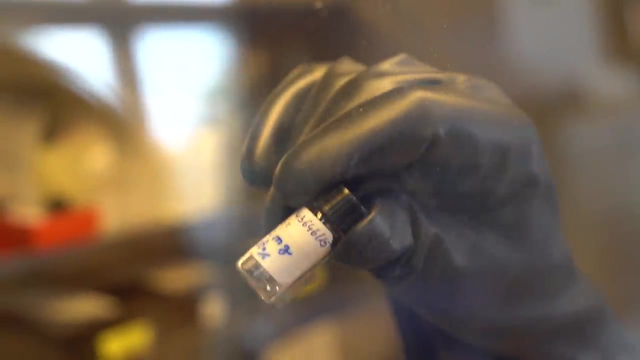 Is there some sure way to increase the cost of gold or some other metals, for instance with some chemical tricks? Hmm, Well, let's find out What is gold. Before talking to you about gold, I would like to consider some other chemicals first, Which can cause hundreds and even thousands of times more than the chemical elements they were made of.